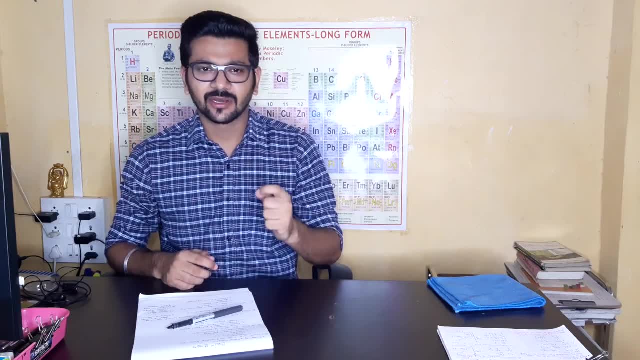 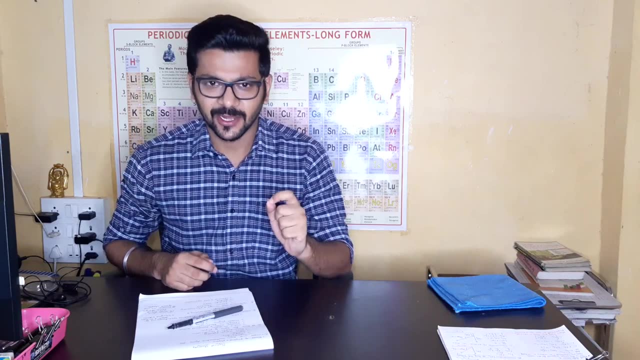 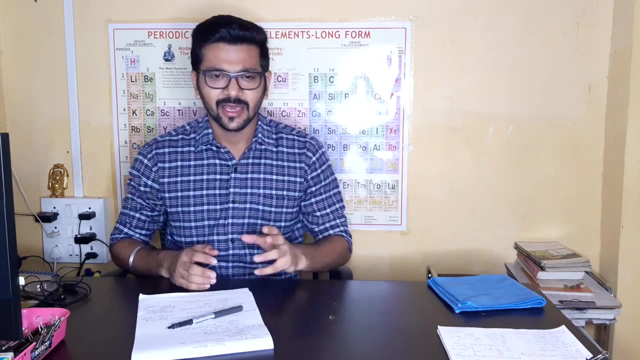 understanding them by hurting them or imagining them. and then let me tell you, then physical chemistry is a nightmare for you, because physical chemistry is not about by hurting. physical chemistry is all about understanding. physical chemistry is all about imagination. in case, if you study electrochemistry, if you're studying thermodynamics, if you're studying chemical kinetics, you cannot. 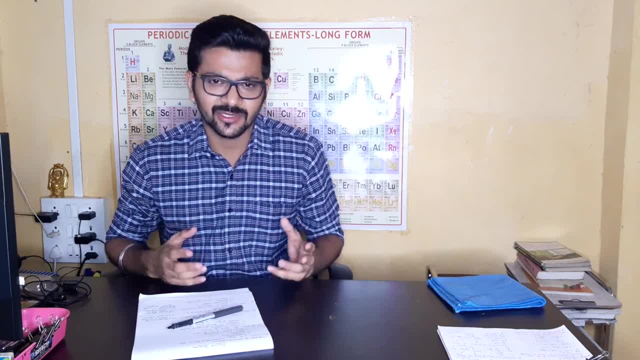 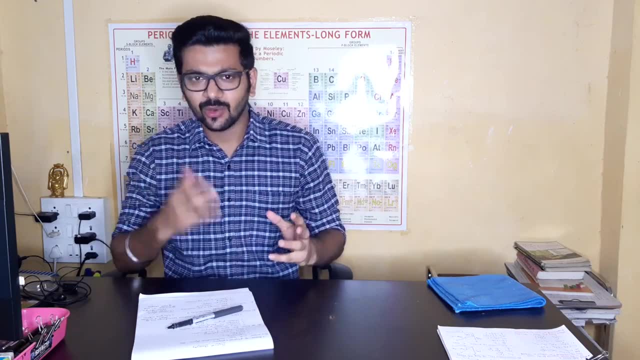 mug up everything. you cannot write a long answer because physical chemistry itself is a very short and sweet branch where you don't have long answers, where you have equations, where a huge amount of things, on one hand, if you have got a organic chemistry and on the other, if you have got a 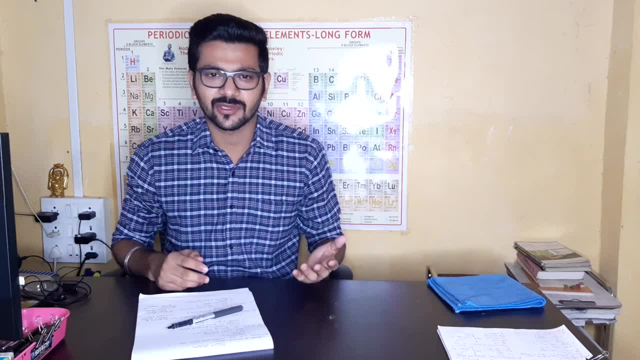 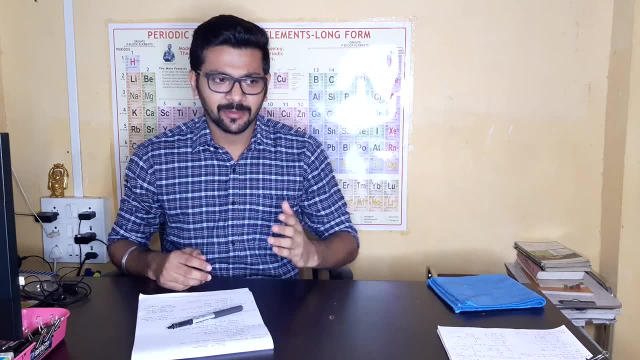 chemical chemistry may require two pages, but a typical answer in physical chemistry will not be more than one, more than a half page. so physical chemistry is something which you need to understand. now let me tell you, being a physical chemist, I can. I can tell you one thing very frankly. 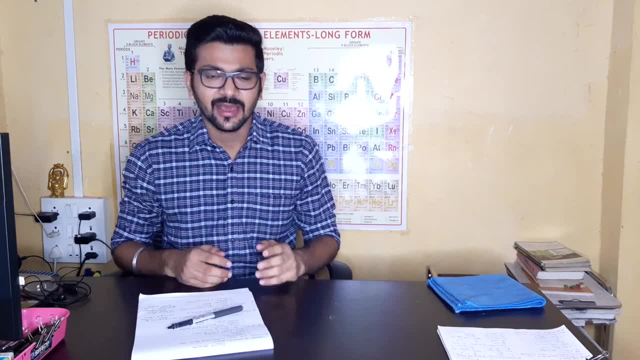 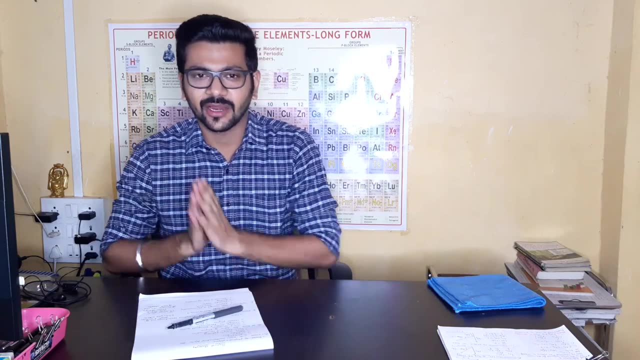 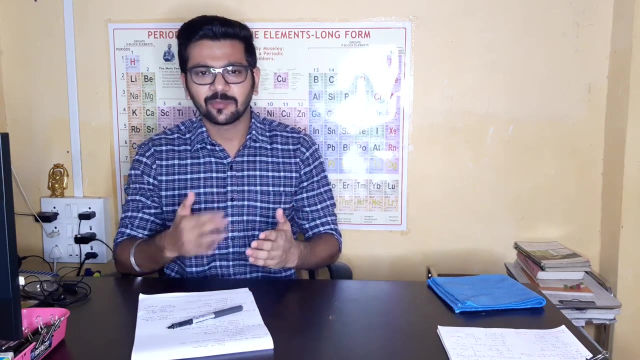 I never buy out physical chemistry. trust me, I never buy out physical chemistry. but there's one more important thing: if you are reading physical chemistry, reading physical chemistry may take more time than reading organic chemistry. organic chemistry or inorganic chemistry is just like, will be just like turning the pages and understanding all the thing by hiding, mug up or mugging up all. 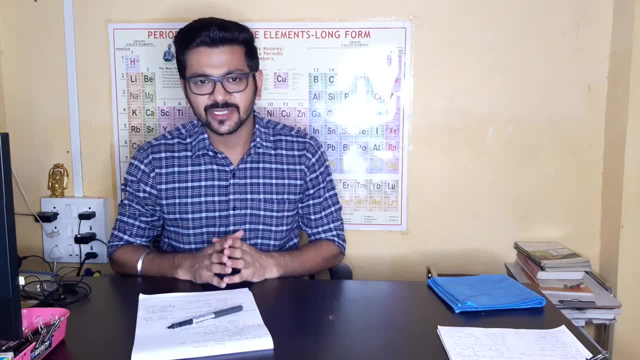 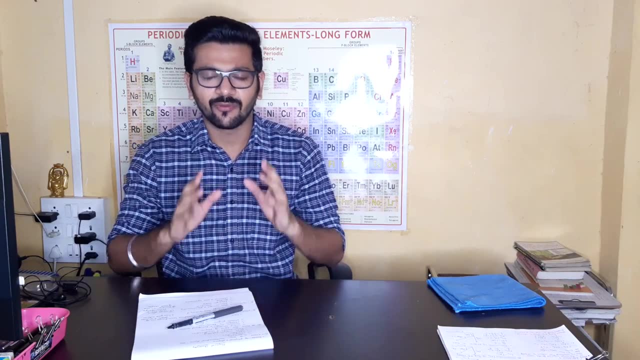 those things but physical chemistry. it may happen. one page of physical chemistry may take one or two day. you may not move ahead from one page. the reason is understanding physical chemistry involves a lot of basic understanding. now many a times students find it very difficult to understand physical 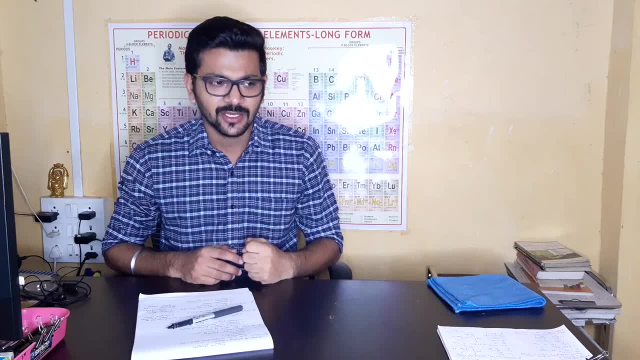 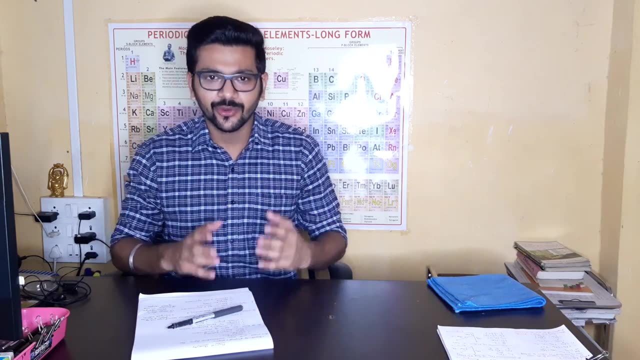 chemistry or to to get good hold on physical chemistry. so from where should we start? so I have got six mantras for you, or you can say six tips from my side from where any student who's learning physical chemistry or who's aspiring to learn physical chemistry should start from. so the 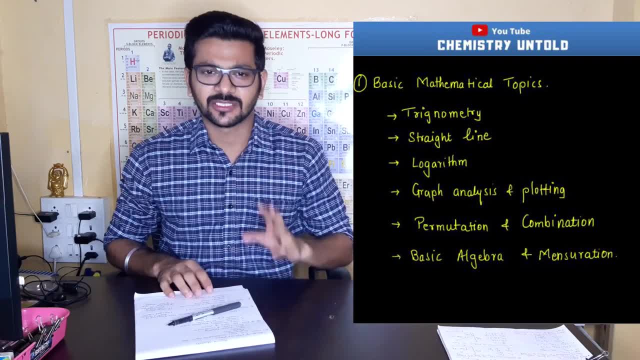 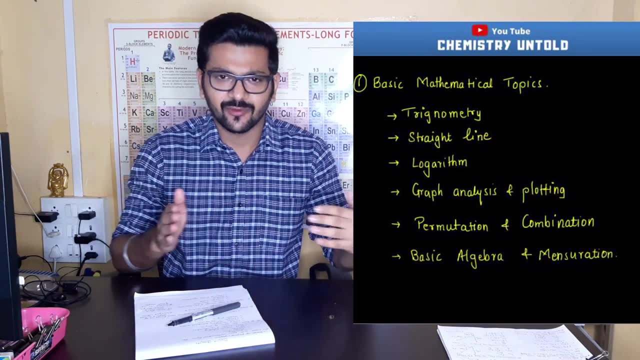 first tip that I'm going to give you is: start with some basic mathematical concept. now we all know. up to 12th standard, up to our 12th grade, we all study mathematics. after that, we all get bifurcated into our different, different streams and different, different branches, depending upon your interest. 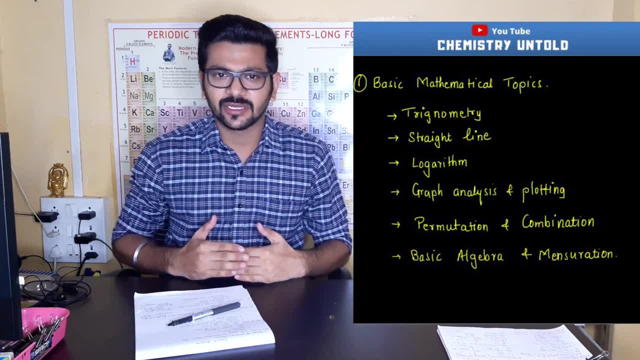 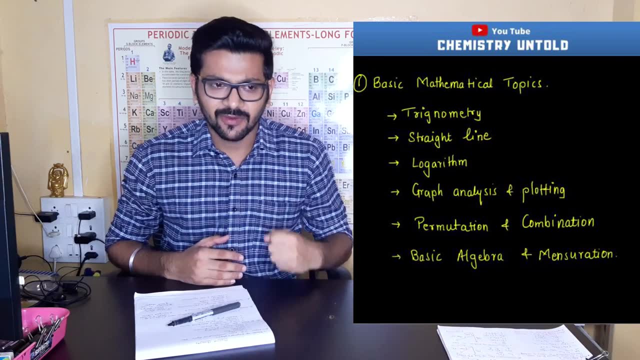 but many a time I have seen this. if if a student really wants to understand physical chemistry, then he will find it very difficult if he is not strong with the basic mathematical concept. and when I say basic mathematical concept I do not really mean that you need to buy hard. higher order trigonometry, higher order derivative. 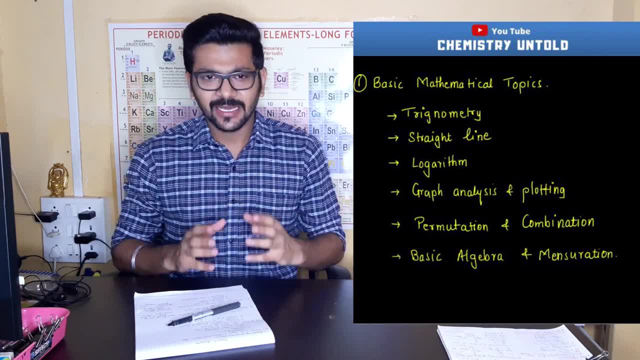 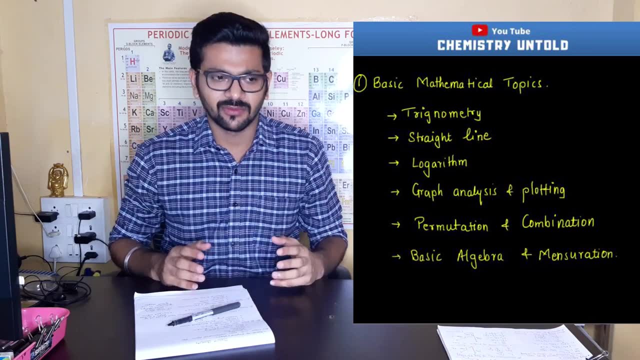 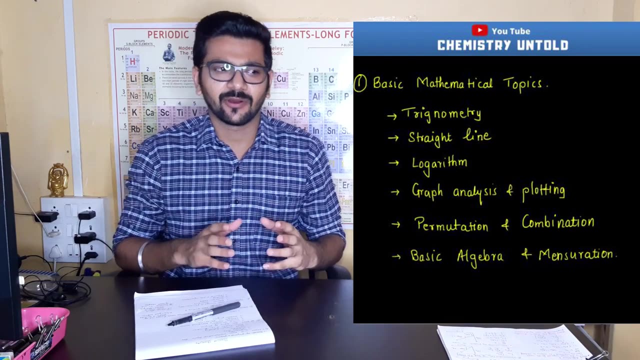 or higher order integration. what I basically mean is the basic mathematics which you have studied till your 12th standard, the basics mathematics which involves straight line, which involves a logarithm, which involve trigonometric functions, which involve algebraic indices, laws of indices. the basic mathematics which was there from your, from a local classes 9th and standard taking. 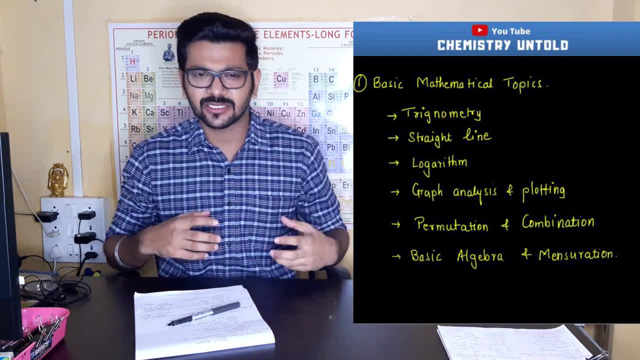 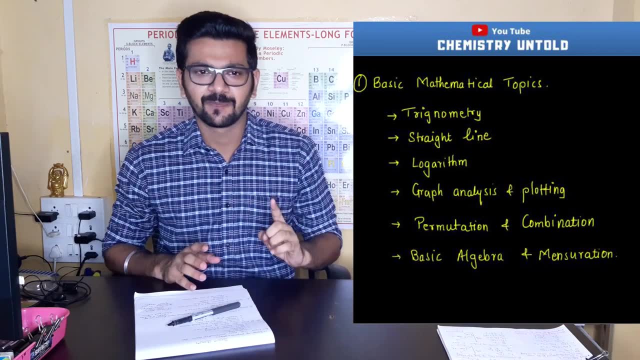 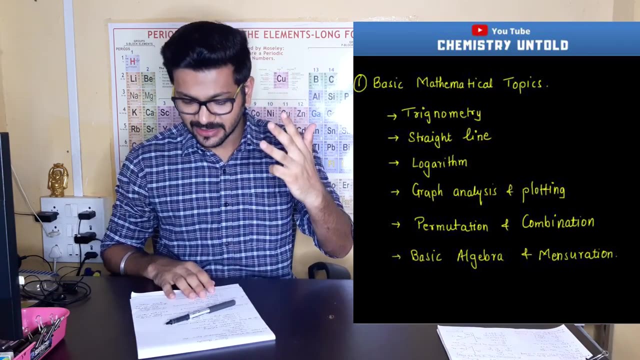 square root, taking squares, taking cubes, solving a complex logarithm by simplifying it. so these are few things. if you master all those things, so you are crossing the first hurdle in understanding physical chemistry. so from where you should start? you should start from trigonometry, straight line logarithm, graph analysis and plotting, because if you know how to plot a graph of a sine, 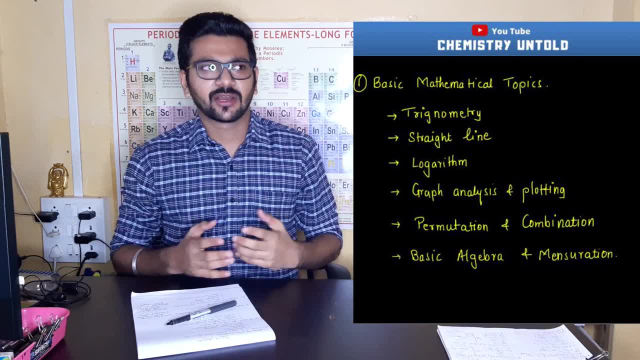 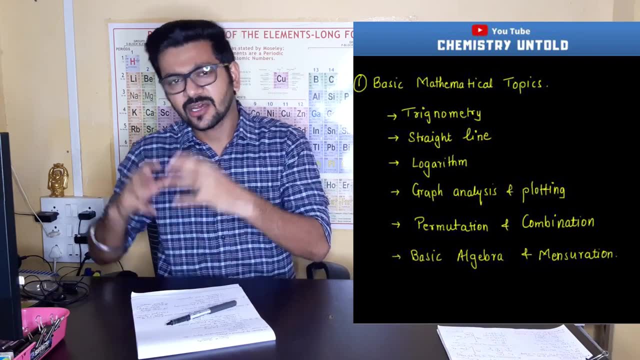 theta. if you know how to plot a graph of a cos theta and if you know how a how a graph of a minus sine theta looks like, it becomes very, very simple. or it becomes very easy for you to grasp the the vast information in the formulas of physical chemistry again. 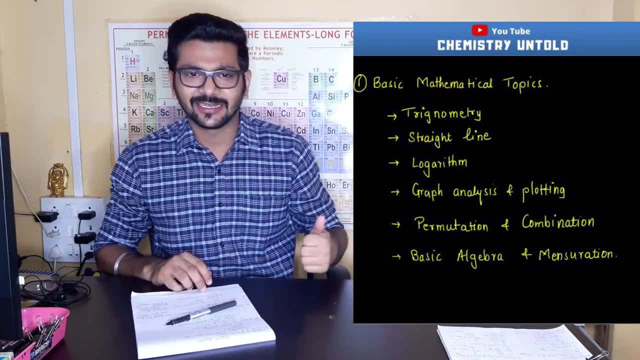 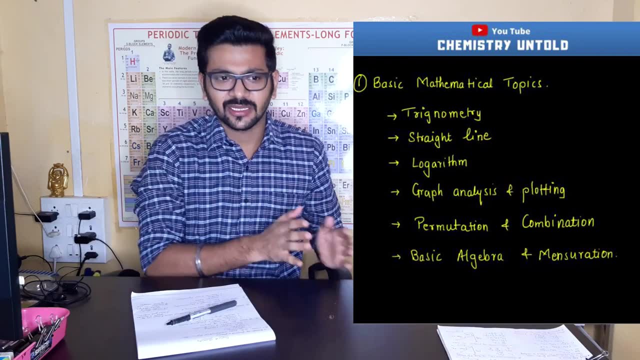 know. and if you don't understand by sine theta, cost theta, tan theta, what are the, what are the graphical interpretation, how do you plot a graph, what does this slope means? and if you don't know all those things, then it will become really difficult for you people to understand physical. 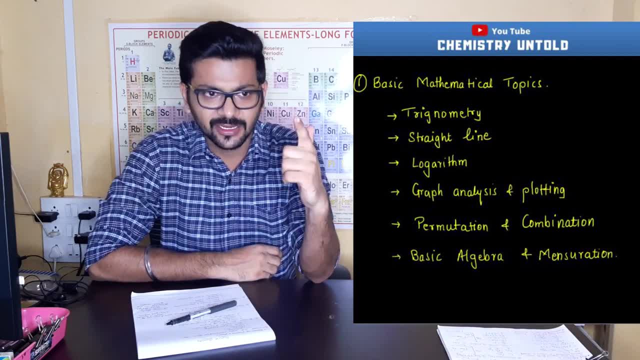 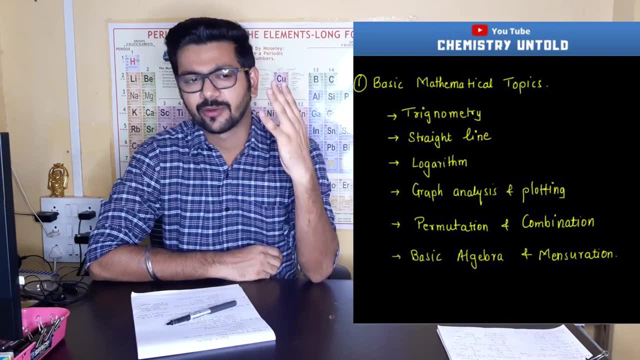 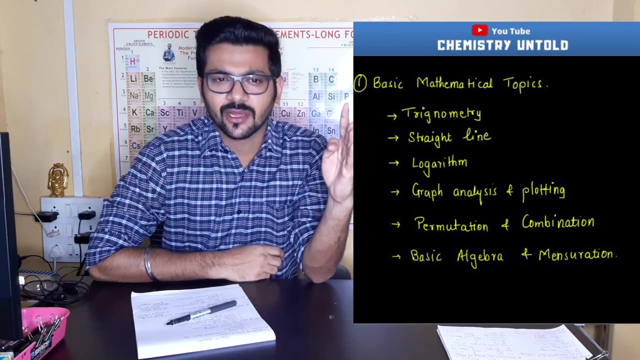 chemistry. so the first thing is you start with trigonometry, start with straight line by heart, the basic formulas of straight line, logarithm, graph analysis and plotting, and the fourth will be permutation and combination. now let me tell you, permutation and combination is for all those people who really want to study thermodynamics, quantum chemistry and statistical thermodynamics. 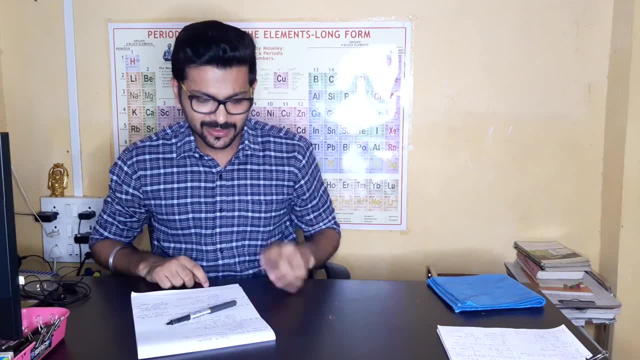 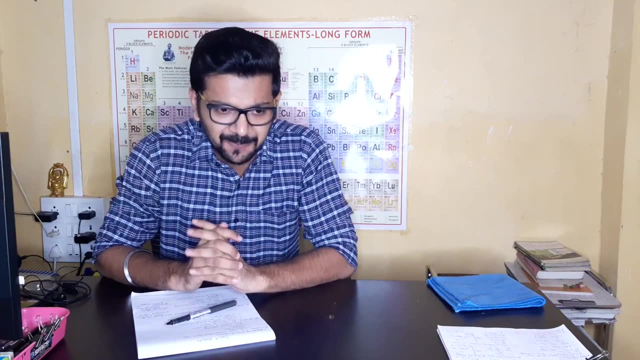 in higher classes. okay, the second mantra that i can give you is: after you cross the first hurdle, that is of basic mathematics, try to practice them now. many times i have seen people telling me that so, uh, we cannot solve the numericals of physical chemistry. you know the main problem behind this. 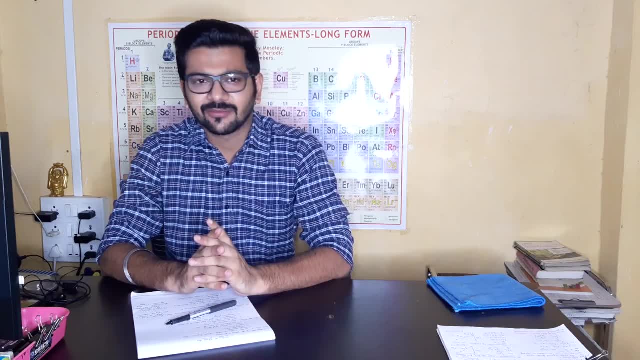 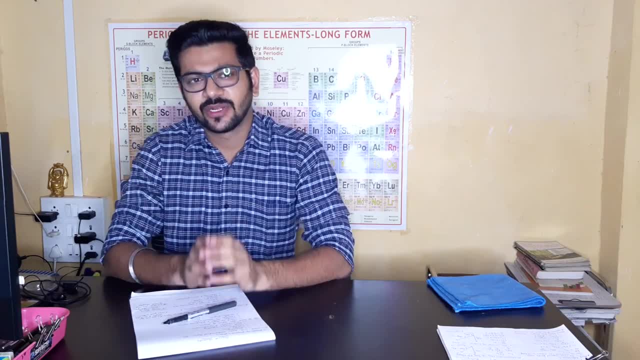 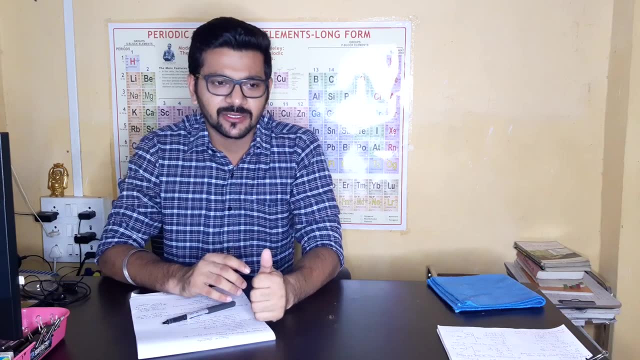 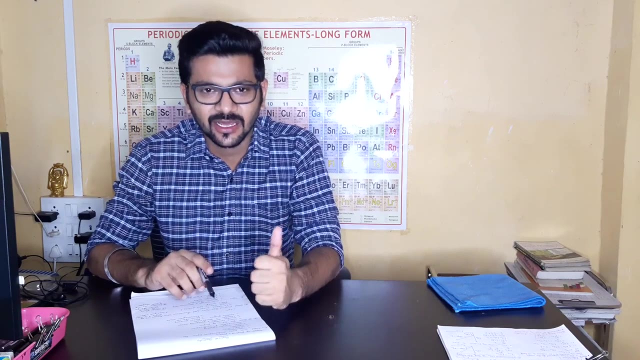 it's very easy. solving 15 into 5 is again very easy. solving 15 into 26- again easy. but multiplying 333 multiplied by 646 is difficult. so the best advice that i can give you is open up your youtube and type vedic mathematics. just watch two or three videos where you can learn how to simply multiply. 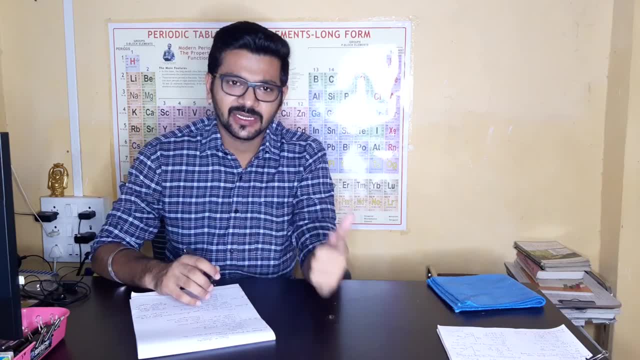 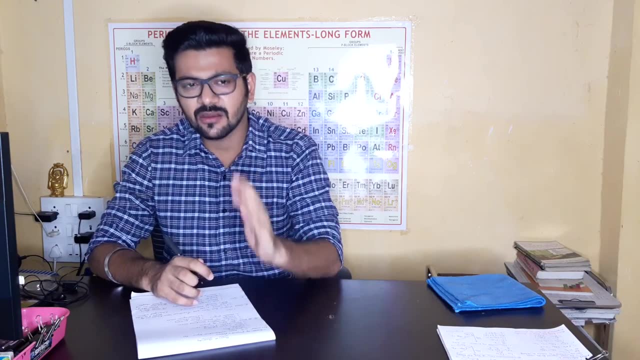 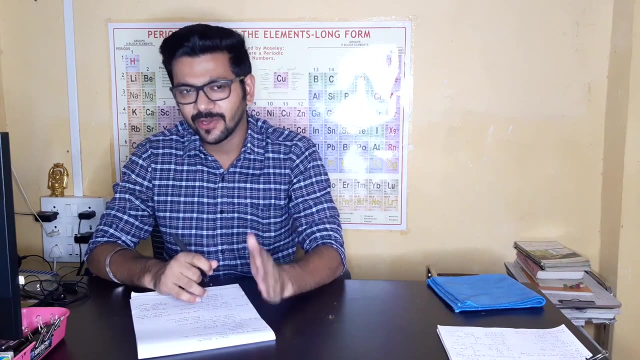 how to simply divide the numbers, and if multiplication and division is on your fingers, probably after seeing numericals, you may not get afraid of it. the basic reason or the main reason why people are usually afraid of physical chemistry is because of the lengthy calculations that are involved and because of the numericals that they have to solve while solving physical 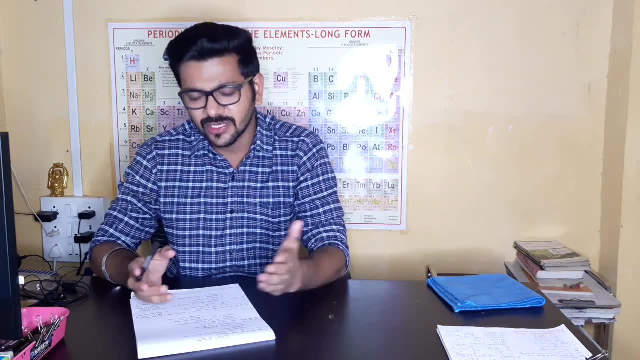 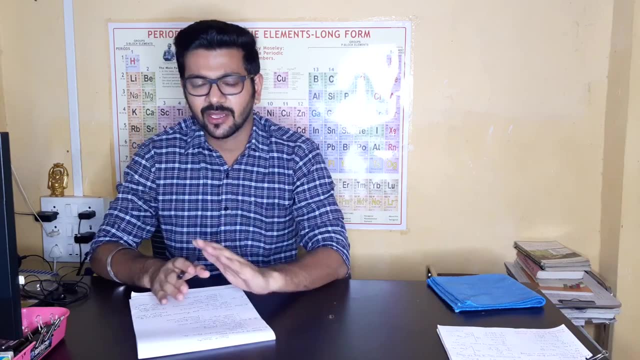 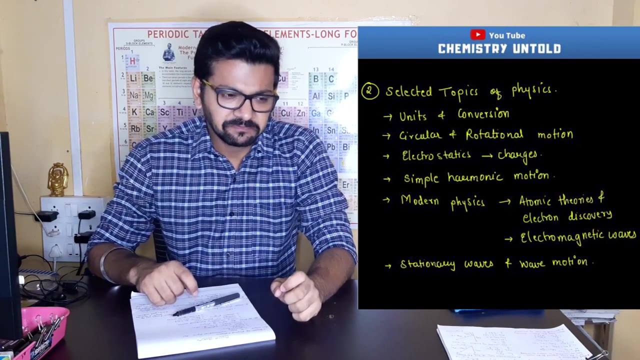 chemistry, and that's probably the reason why people start, all the students start avoiding physical chemistry. and let me tell you- i have already mentioned it- physical chemistry without physics and mathematics is incomplete. trust me, it's incomplete. okay, now, once you are done with the basic mathematics, the next hurdle will be physics. well guys, let me tell you very frankly: 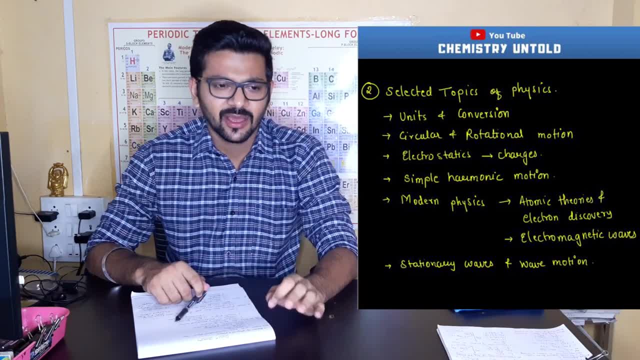 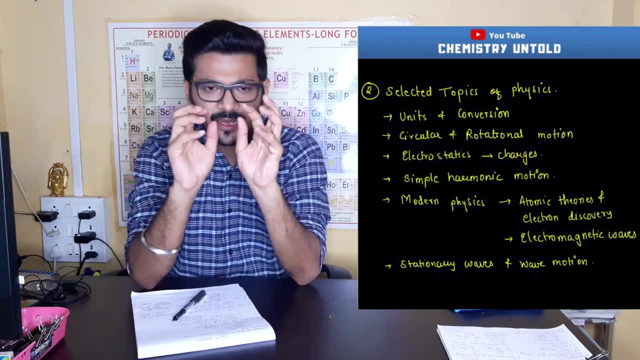 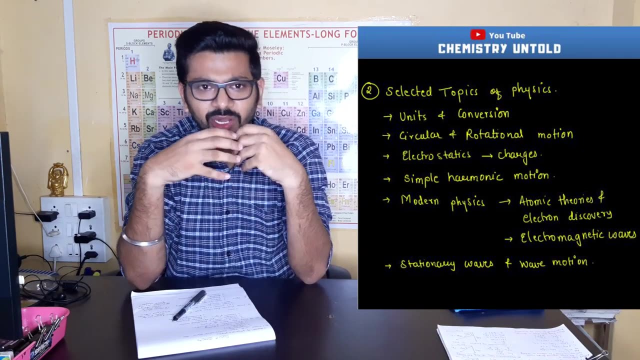 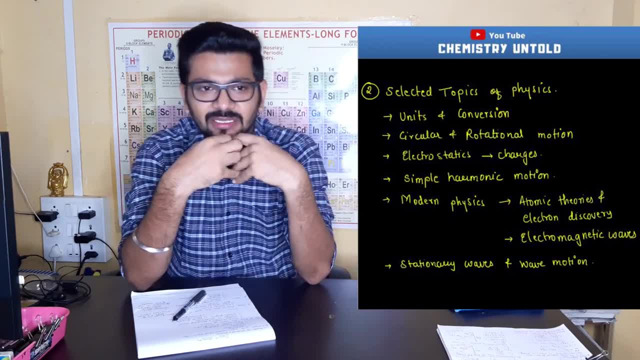 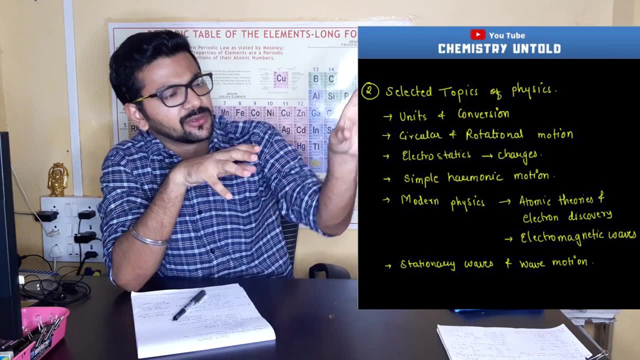 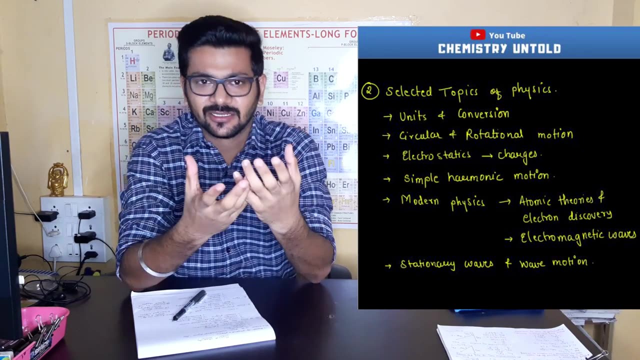 is a feeling that you have got inside you, but expressing it in words that i love you, is a language. so if there is some phenomenon going on and if i'm observing it, observation- doing an observation- is physics. the phenomenon occurring over there is physics. okay, there's a phenomenon occurring over there, but expressing it- 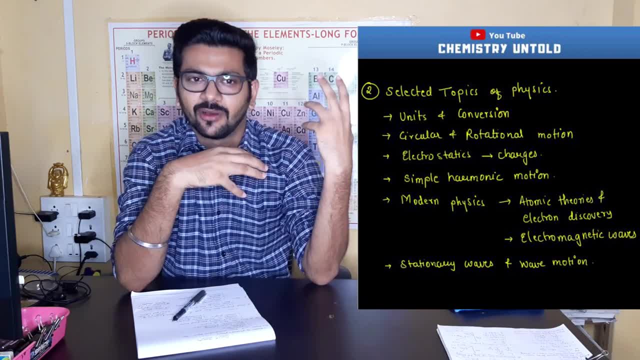 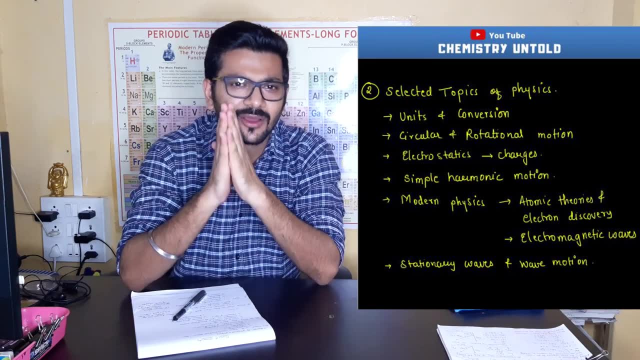 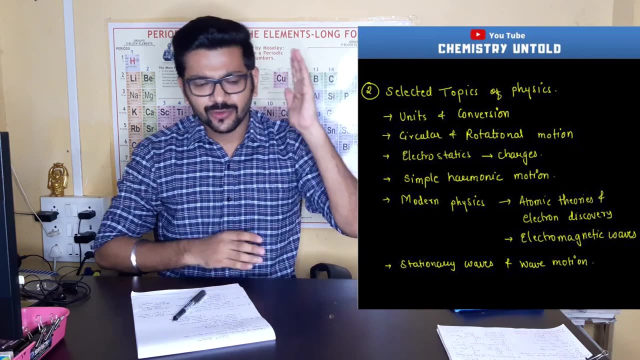 and deriving some equation so that i can play with that phenomenon anywhere throughout the world is mathematics. if you are not good with mathematics, you may miss the beauty of physics and the beauty of chemistry. so in order to understand physics, you should know mathematics. so start reading physics. 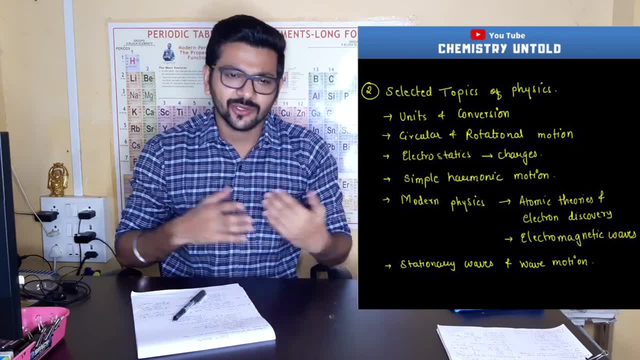 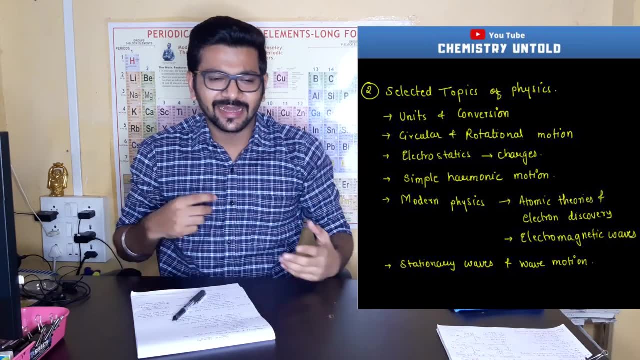 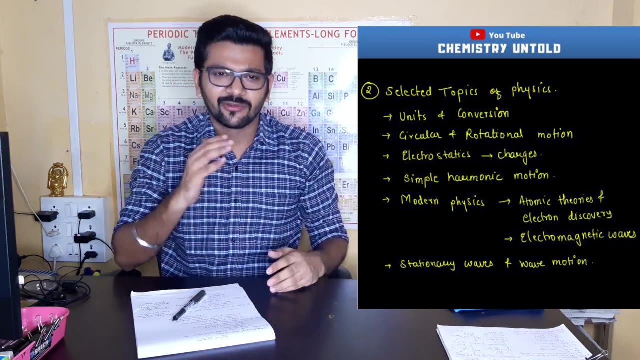 after your mathematics is completed many times. what students usually do is they start with physics and then, when they find it tough, they don't understand the uh, the formulas, they don't understand the derivative, they don't understand the graphical interpretation, and then they start hitting physics. and if you start hitting physics, obviously i can bet you that you will really hit. 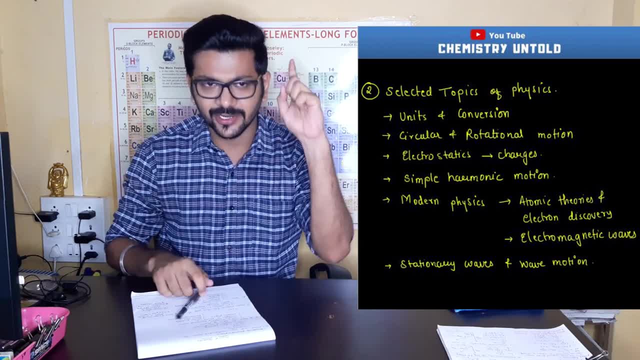 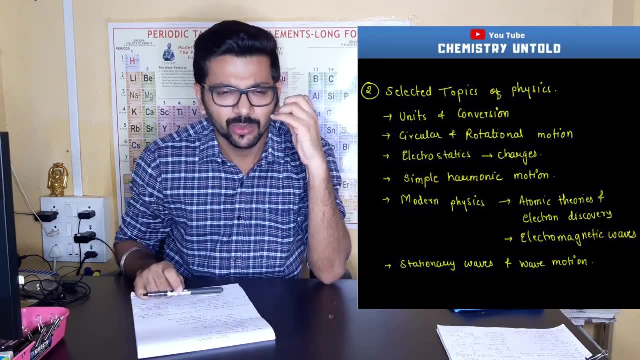 physical chemistry as well. okay, so start reading physics. what are the topics that you need to read in physics? start with units and conversions. you know- many times i have seen people from chemistry background- that they are very, very weak with units. they are very, very, very weak with unit conversions. 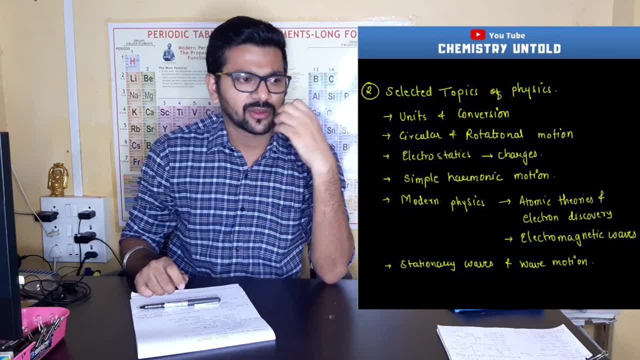 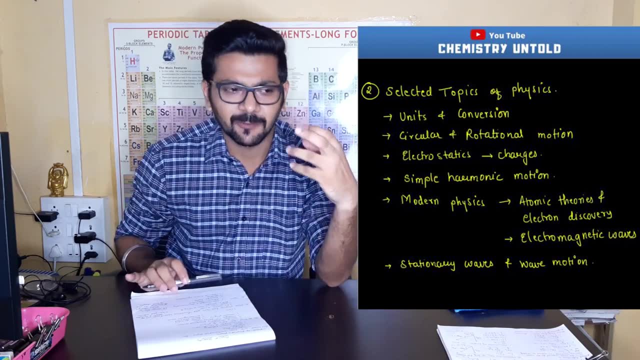 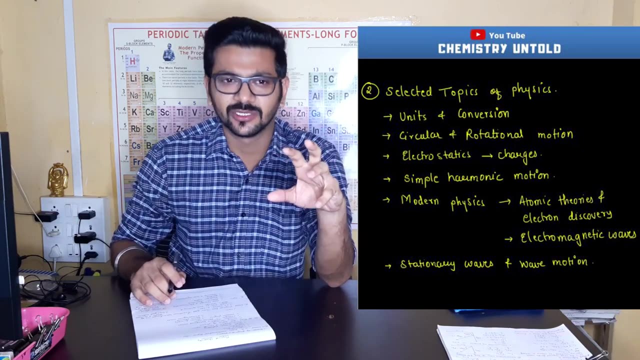 like if there's milligram conversion, from milligram to gram, for from kilometer to meter, from angstrom to picometer, from centimeter to nanometer. students find it really, really difficult the conversion between the different values of energy, joules, electron volt. you need to start by hurting all those units and conversion, all those units and conversions which. 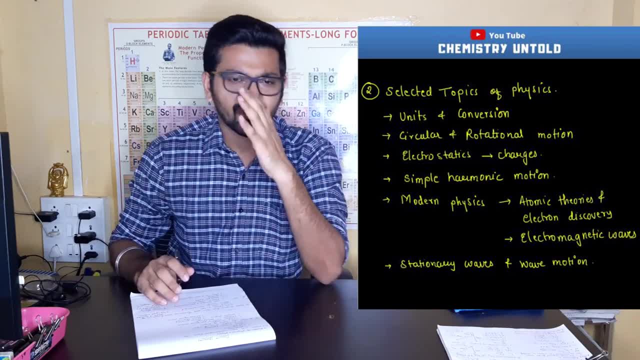 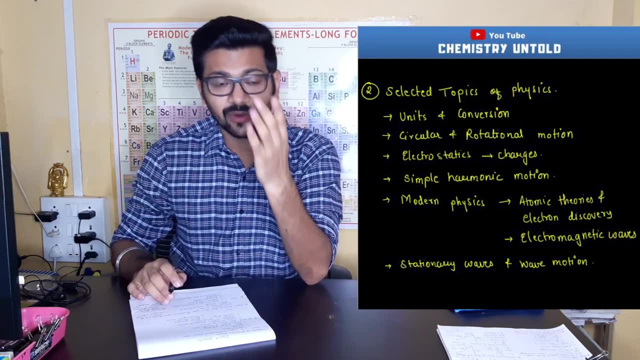 are really, really required for understanding physical chemistry. well, uh, for this i can help you out. i've already made a video in states of matter playlist where i have, uh, where i have introduced few of the unit conversions you can watch. the link for that video is given in the. 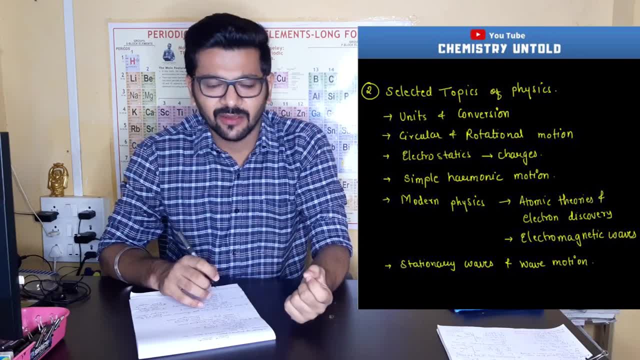 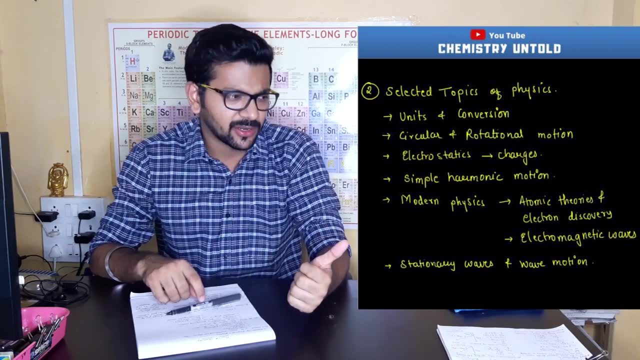 comment box. you can go and click there and you can watch the video. if you want to watch the video, it's a basic video where i have introduced a few of the unit conversions and probably that may help you. okay, then you should start with circular motion and rotational motion. it can be called as rotational. 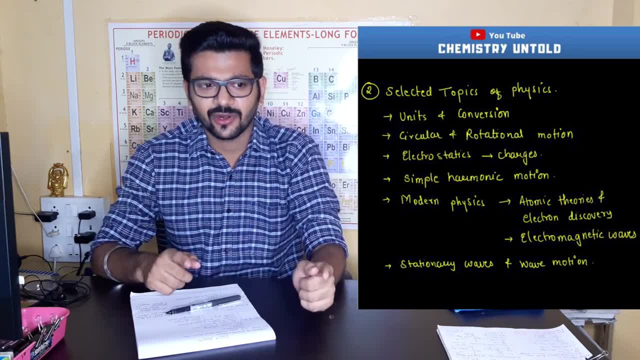 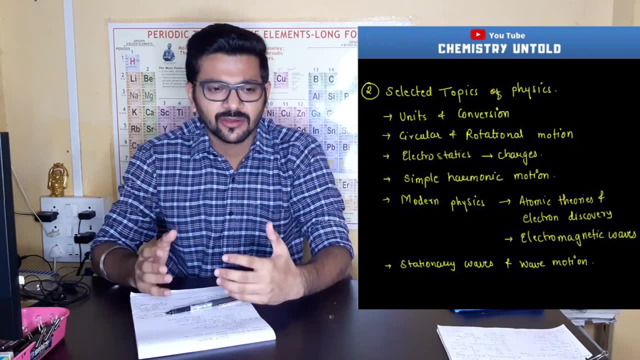 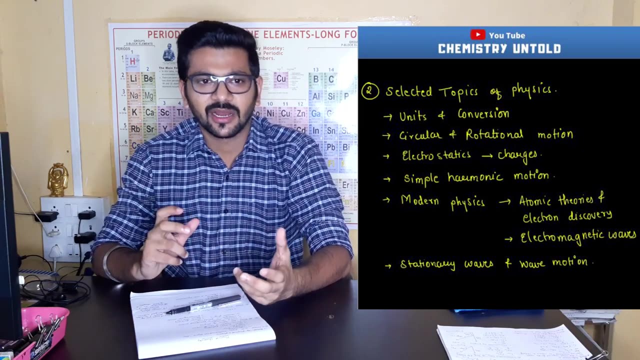 dynamics, circular motion and rotational motion are really important for understanding atomic structure because most of the most of the phenomena that you are going to observe in atomic structure are going to involve circular motion and in spectroscopy they are going to involve rotational motion, molecular rotation, molecular electronic circular motion. and, in case if you are not good or 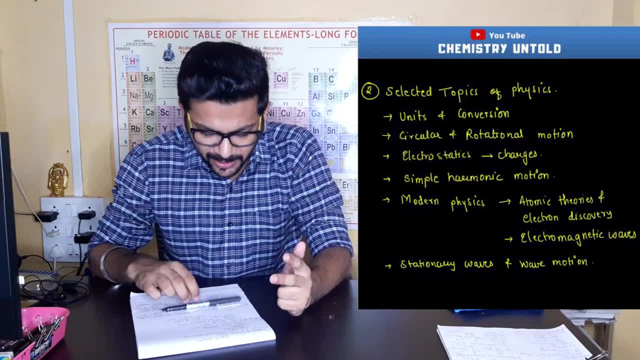 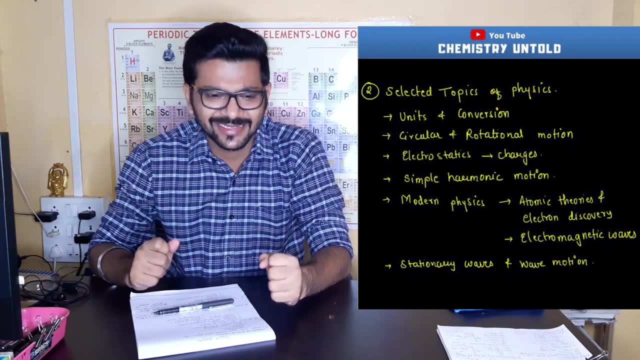 strong with this. you may find it difficult. the third: the third topic from physics that i can tell you is start reading something about um mechanics, mechanics. what i basically mean by mechanics is just having a brief idea about what do you mean by velocity, what do you mean by speed? 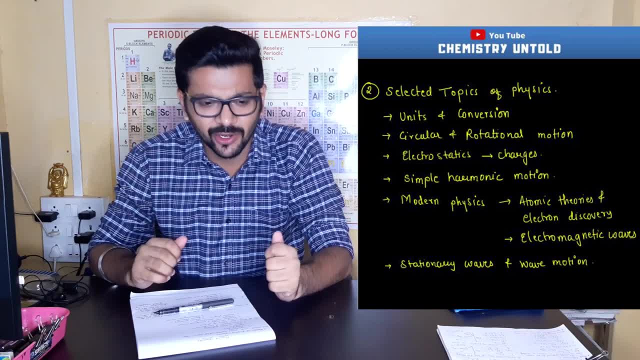 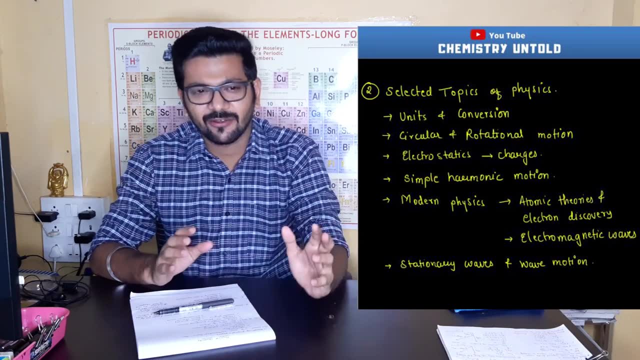 few of the kinematic equations. what do you mean by a derivative? what do you mean by, uh, maxima, what do you mean by minima? and all those stuff from classical mechanics- okay, from classical mechanics. start reading all these things, okay. the next topic will be charge and electrostatics. 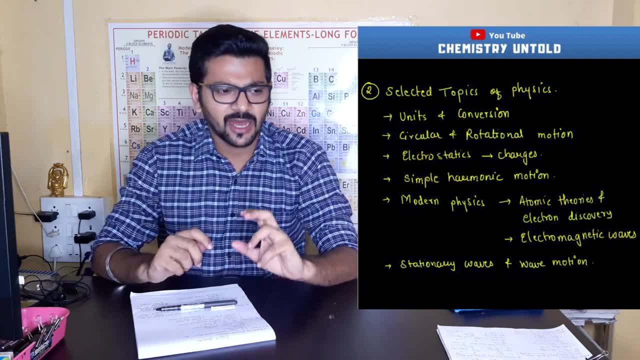 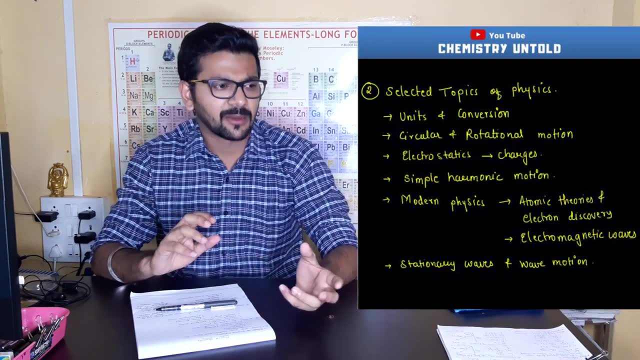 so what you need to do is start selecting information about charges on electron, charges on proton, mass of an electron mass of a proton, the electrostatic force of the electrostatic force of attraction, the formulas for them, about permeability, permittivity. all these things will build up your 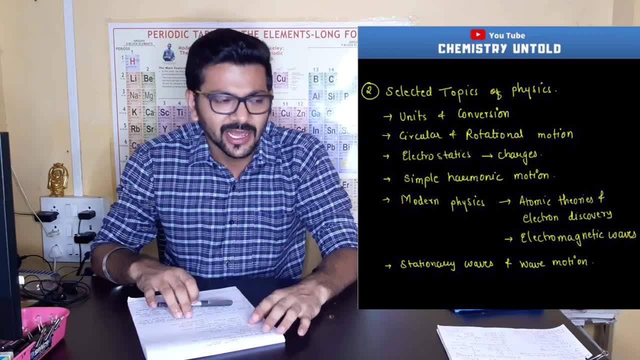 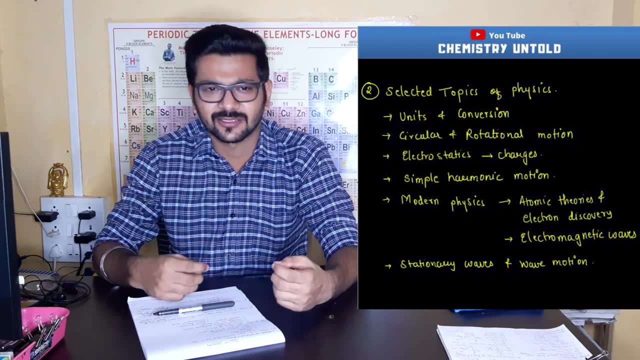 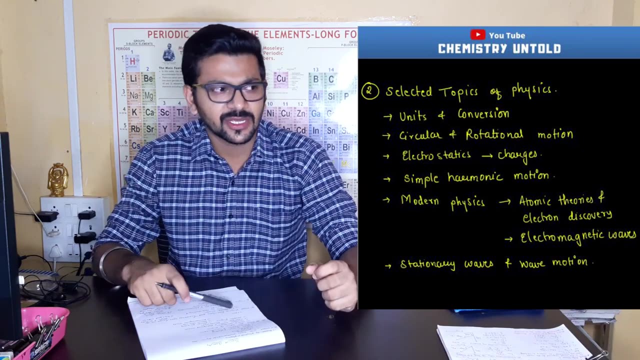 basic in understanding higher order physical chemistry. okay, the next topic will be modern physics. now, what do you need to study from modern physics? you need to study electron discovery. just spend some of your time- few minutes or few hours- on electron discovery. watch some good animated, try to understand them. note down some important points from those videos. what do you learn you? 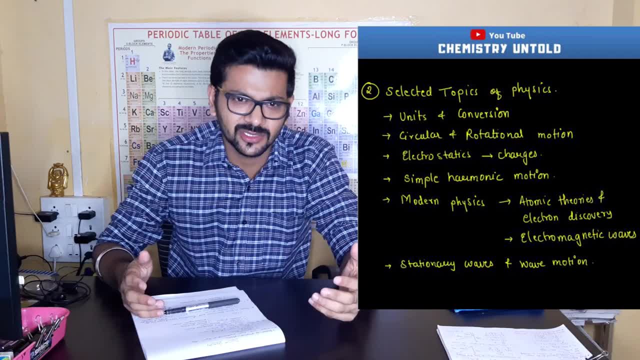 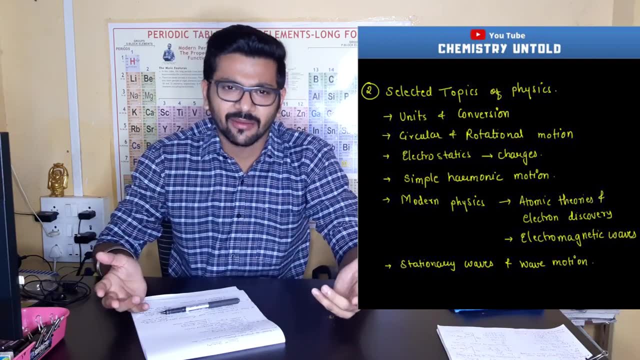 don't need to buy hard which scientist or in which year the electron was discovered and who discovered electron? who gave which theory. you should know the theory, even if you don't remember the name of a scientist. it's, it's okay. it's okay. well, you should know. but it's okay, it's not going to affect. 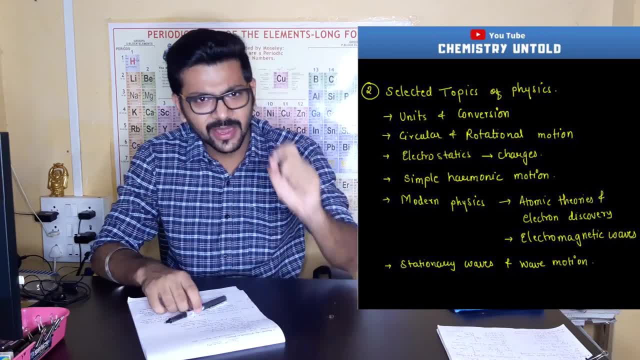 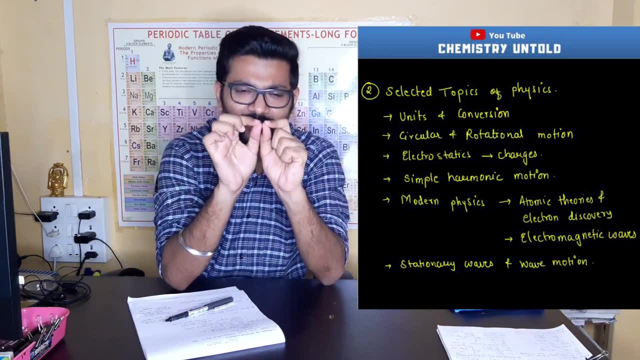 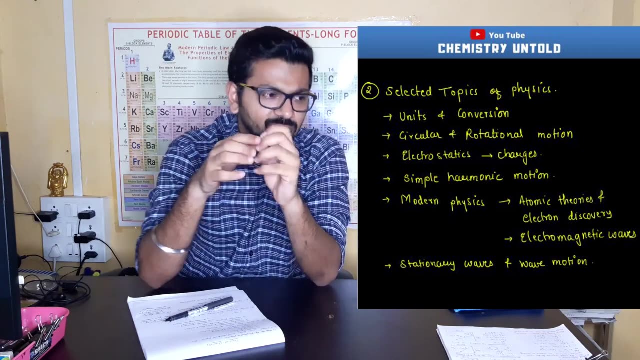 your knowledge. okay, then start with atomic theories. you know the basics of chemistry is atomic structure. the place where physics and chemistry meets is called as atomic structure, and where physics ends is atomic structure and where chemistry starts is atomic structure. so you can say atomic structure is the interconnection of, the link or the bridge between physics and 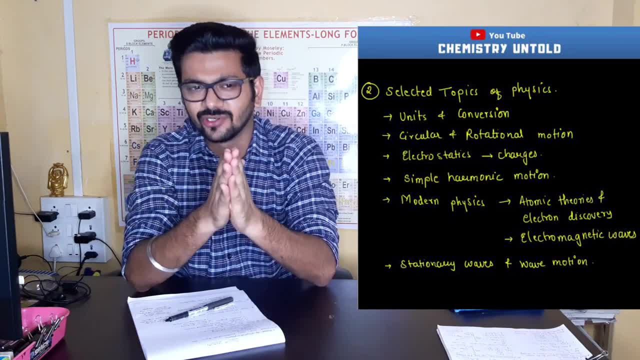 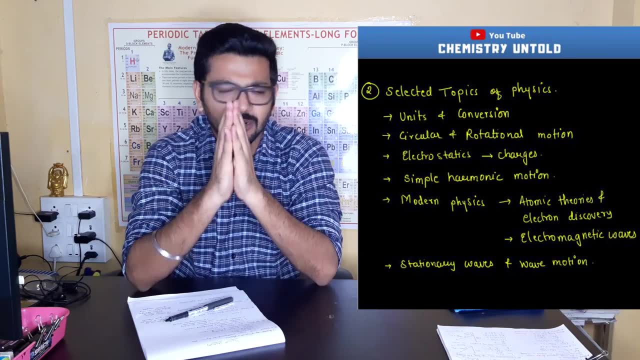 chemistry and in in any case, if you are weak in atomic structure and if you are weak with the basic knowledge about atomic structure, let me tell you one thing frankly: uh, by hearting chemistry, or understanding chemistry, will be really tough for you people. so start with theories. many 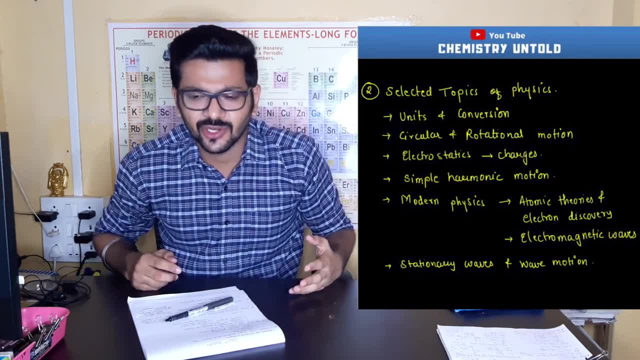 time people ask me: so we are in masters and we are in bachelors, why do we need to study about boho's model? why do we need to study about boho's model? why do we need to study about boho's model, study about rather ford model? why do we need to about all study, about all those theories which? 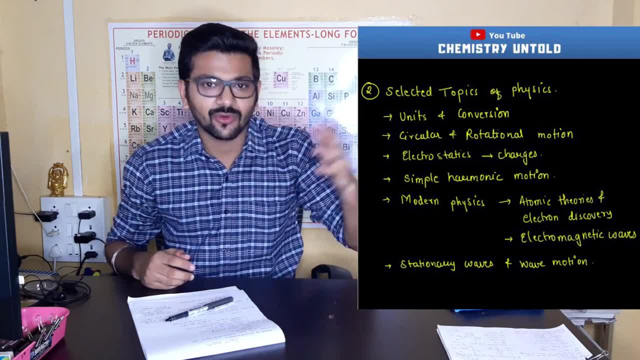 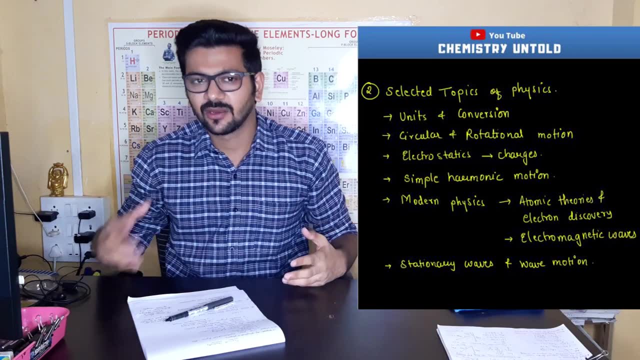 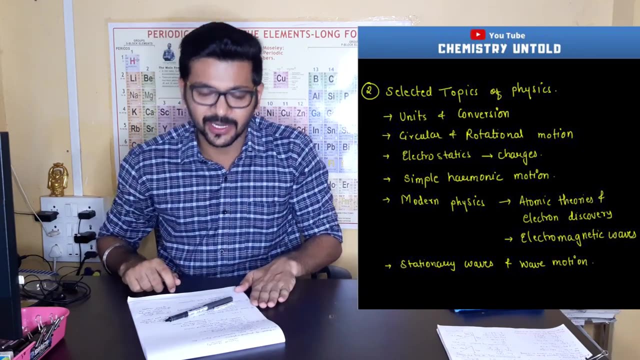 failed. the reason is, when you know what what happened was wrong, you can start discovering something new. if you don't know why that particular experiment failed, you will never be able to discover something new. so you should know why jj thompson's model failed, why another ford model failed, why, why neil boho's model was accepted, why there were some drawbacks in neil. 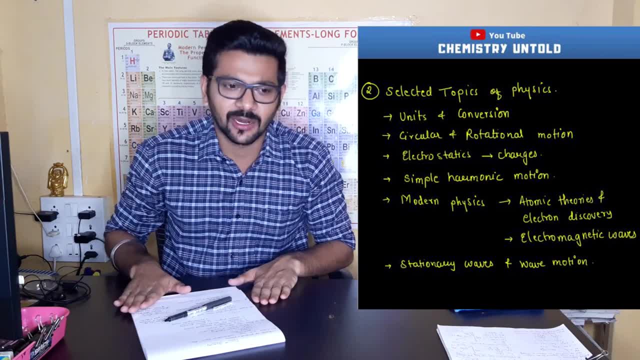 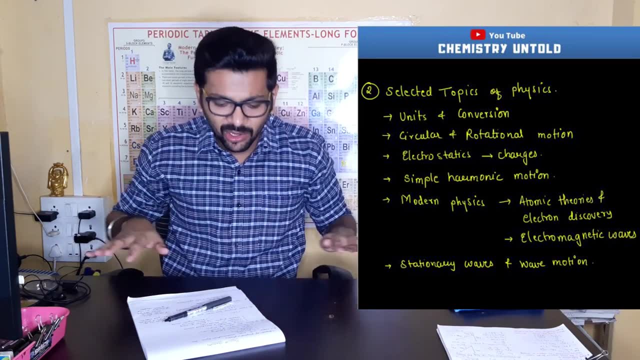 boho's model, why there was a need for, why there was a need for quantum model, what scrodinger did, what was the contribution of d broglie? what was the contribution of of heisenberg? when you know, all these things appeal, your picture about atom is created in your mind and then applying. 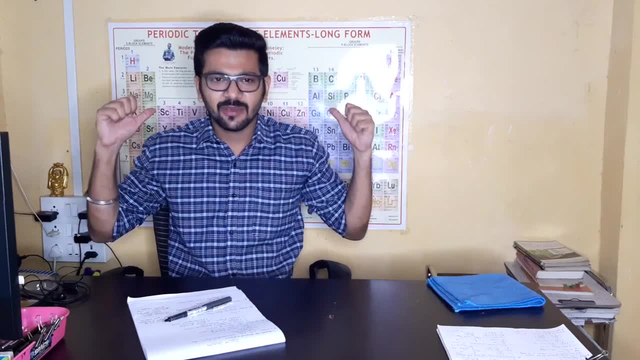 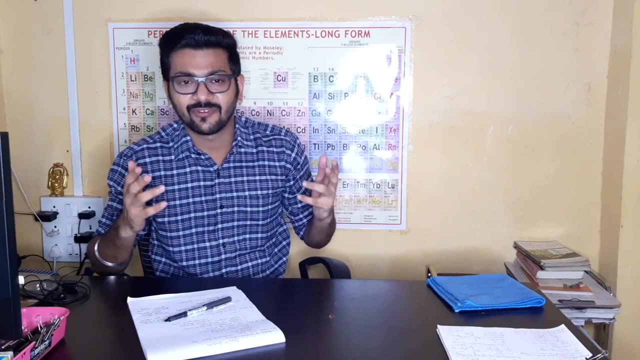 that knowledge on the chemical world becomes quite easy. as you can see, behind me there's a periodic table and there are 118 elements. now, what is element elements are? there are 118 types of different, different atoms, and if you don't know about adam, all these atoms are going to play. 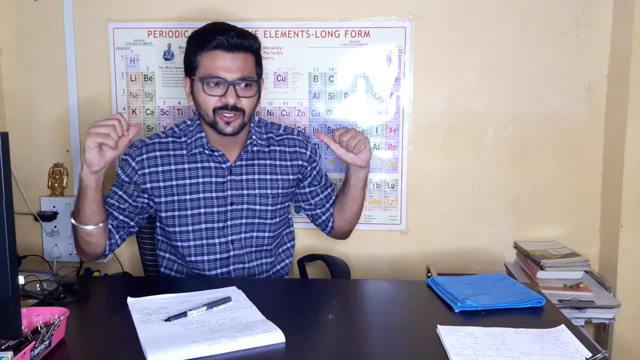 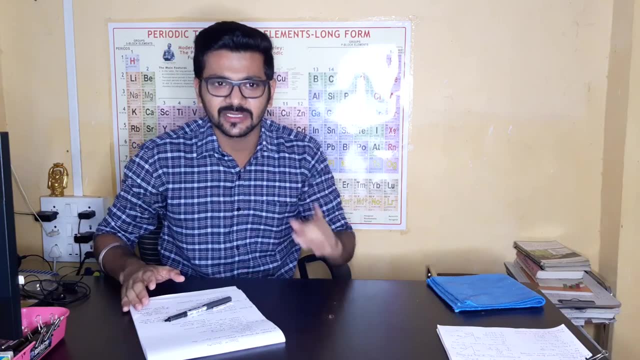 then they are going to create the beautiful chemistry which we can see around the world. so the whole chemistry which is taking place, the sharing of electron, the covalent bonding, whatever you see throughout the universe, is just because of all these atoms. and if you don't know, 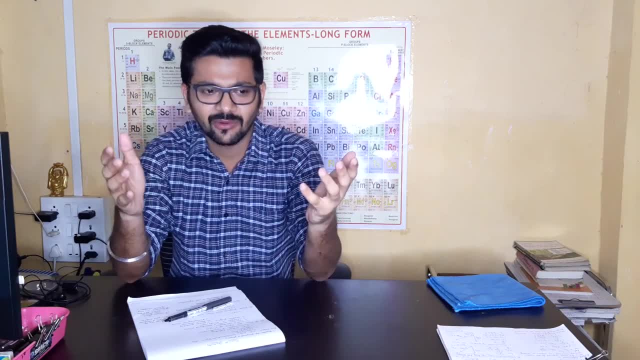 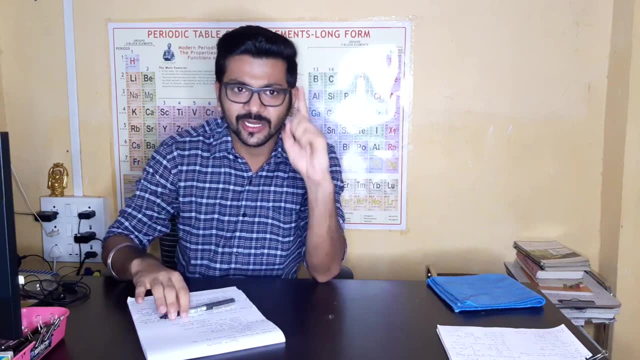 about atoms. it's just like you are watching a movie but you don't know about the main hero, or you don't know about the main character over there, but you are just trying to watch the entire movie. okay, so start with atomic theories. the next will be about electromagnetic waves. you know when you 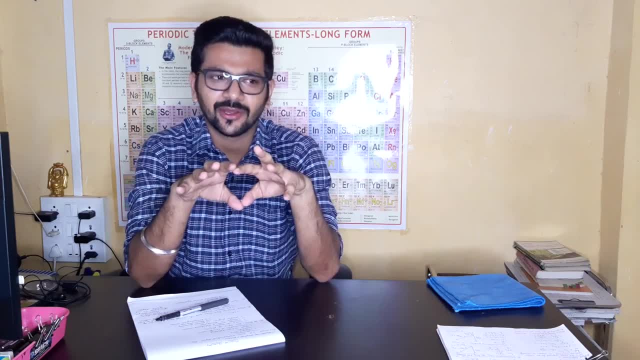 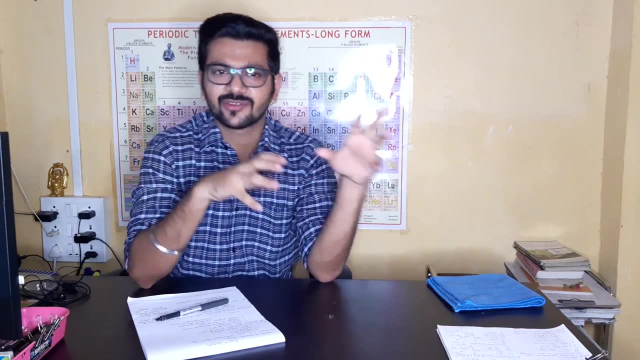 go to higher level, the higher order chemistry is completely dominated with either electroanalytical methods or either spectroscopy. when you go to your masters and when you study the chemistry which is related to industrial chemistry, industrial chemistry involves two chemistry. let me tell you one thing very frankly: one will be your electrochemistry and the other 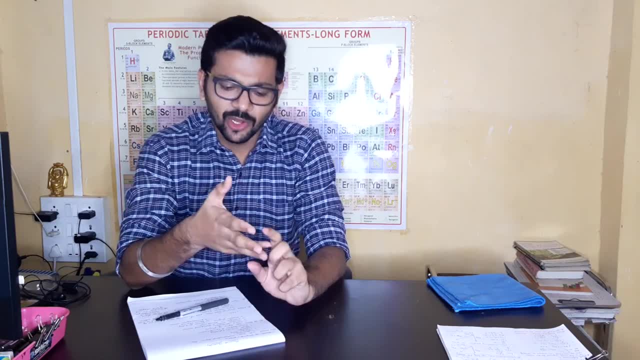 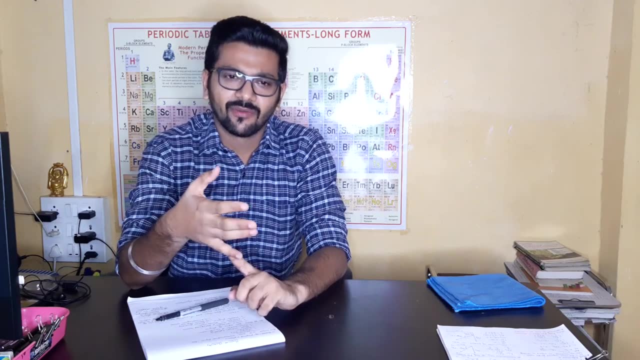 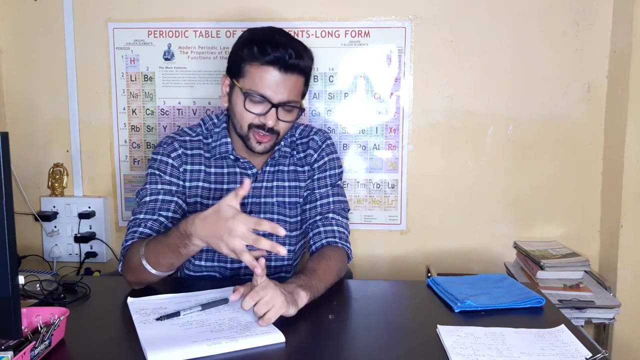 is going to be your spectroscopy, because analysis, molecular elucidation, is going to involve spectroscopy and when you deal with industries, the analysis is going to involve electrochemistry. so these two are the branches, and both the branches are some of the other way. especially, spectroscopy is going to deal with electromagnetic radiation and matter, whereas electroanalytical 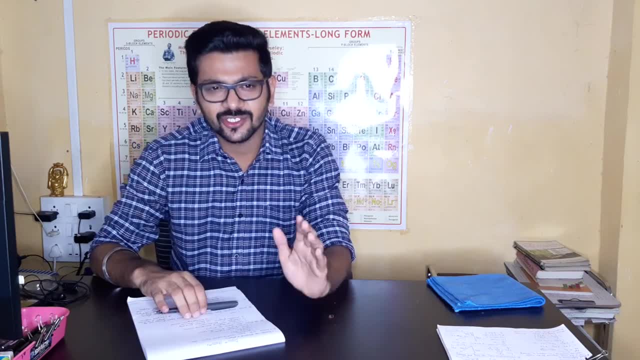 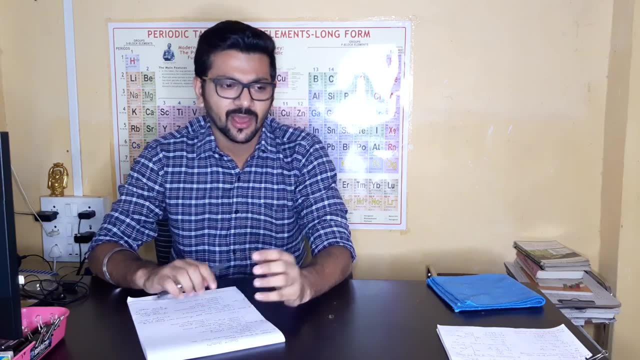 method is going to deal with current electricity. you should be quite strong with electro, with current electricity, in case if you, if you are not aware or if you don't have good, proper information about what do you mean by emf, what do you mean by voltage, how the current flows, what actually 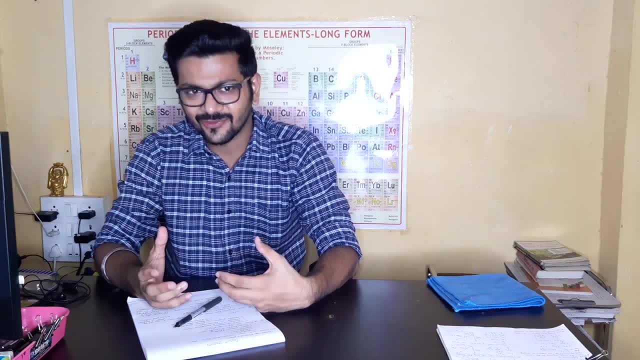 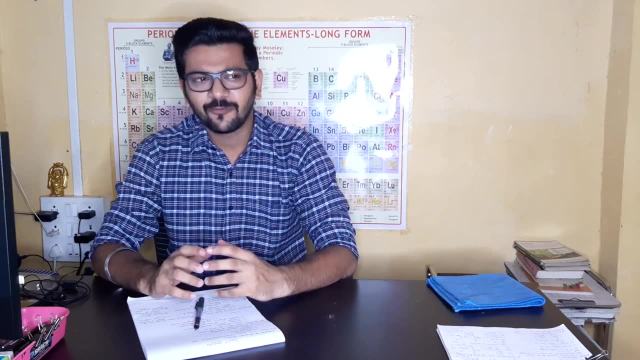 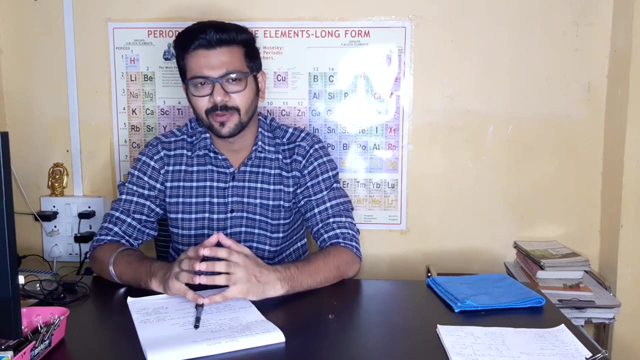 is current. what's the difference between uh, the conventional current, and the real current that is flowing inside a conductor? how does the resistance work- resistance in parallel resistance- and how does it work in parallel? so, in terms of the current flow, you will find it difficult to understand electrochemistry- and electrochemistry is one of the vast topic and one of the largest. 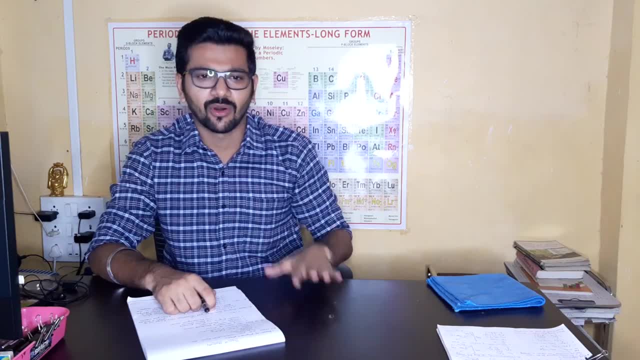 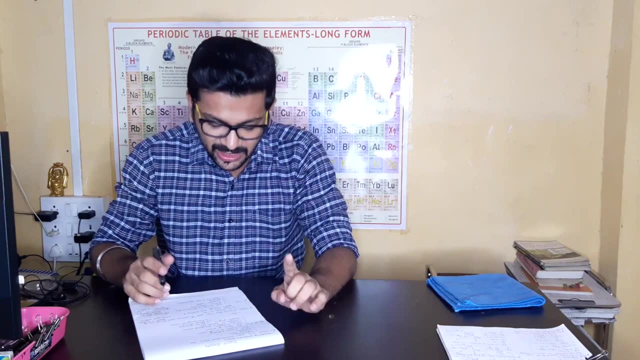 topic in in higher chemistry that you're going to study, so start preparing for current electricity from now onwards. okay, this is the second mantra that i can give you, even though it was a lengthy mantra. the third mantra that i can give you is about start reading some good reference book. many 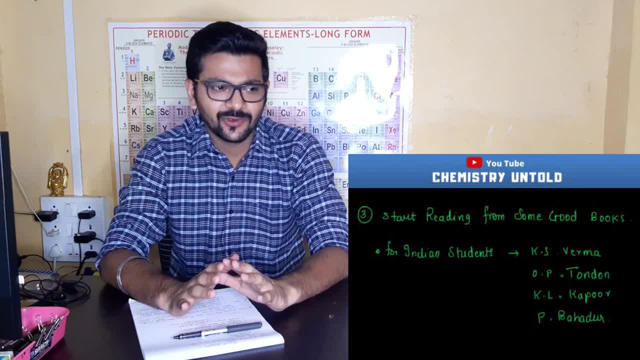 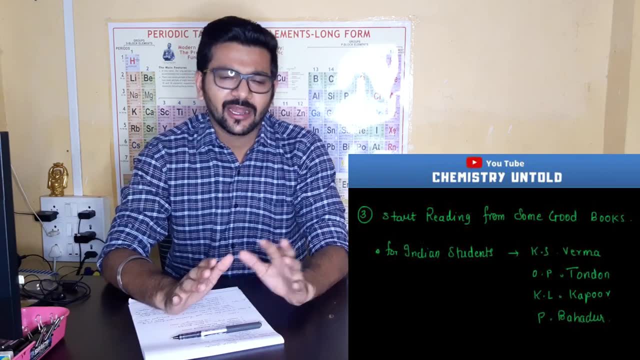 times i have seen people depending entirely on their in their academic books. especially if you are in your eighth, ninth, tenth or eleventh, twelfth, the the students usually have a tendency to depend entirely on their academic. look, let me tell you your academic books that you are going to read in your 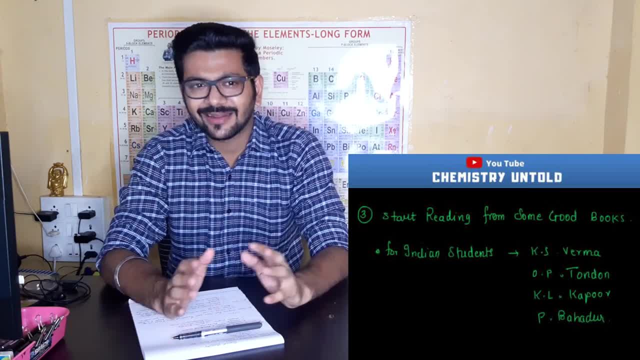 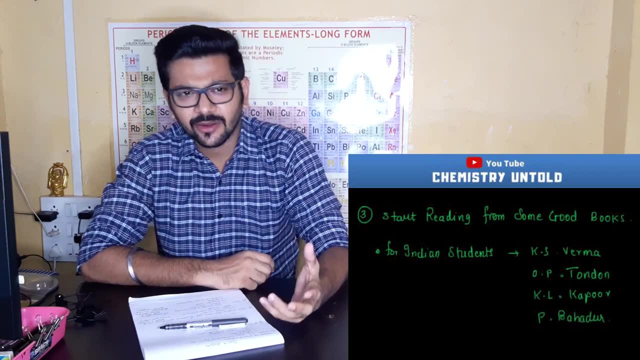 colleges or in your schools will may not be covering the entire syllabus in that particular case, you need to start reading some good reference book. okay, you can find many of the good reference books in the form of pdf. on google you can search for good reference book. uh, you make use of youtube. 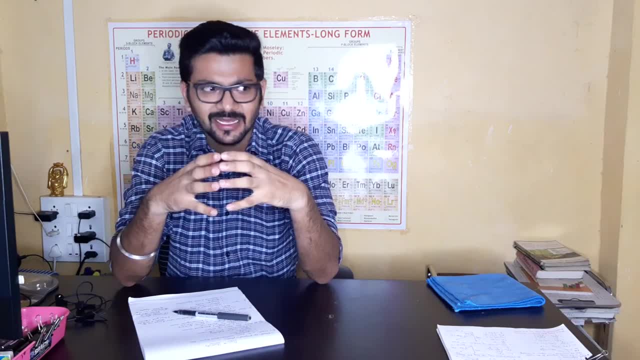 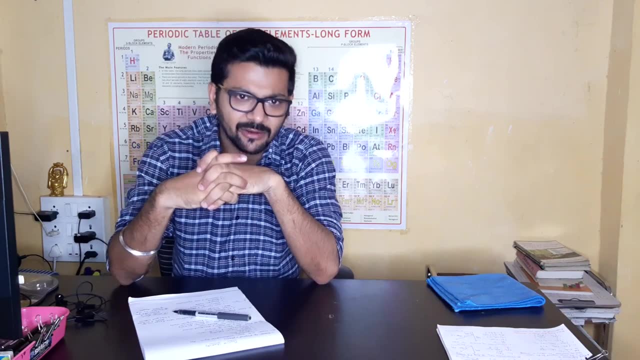 and make use of google websites. there are few good websites. the link of those websites i have given in the description box you can check them. these are the website which i usually refer for clearing my doubts, in case if i've got some basic doubts in any of the basic topic, i usually go to these two websites. one is for physics and the other 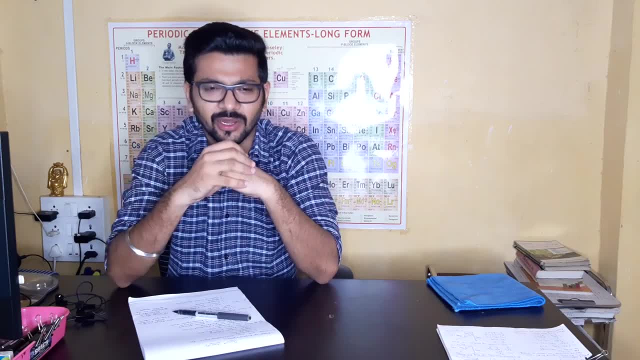 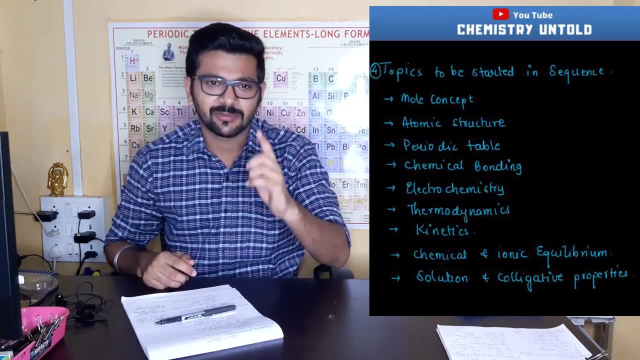 one is for mathematics. i've given the link in the description box. you can go and click over there. the fourth mantra that i can give you is: start with mole concept and stoichiometry. trust me, understanding mole concept and stoichiometry is the primary requirement for studying physical. 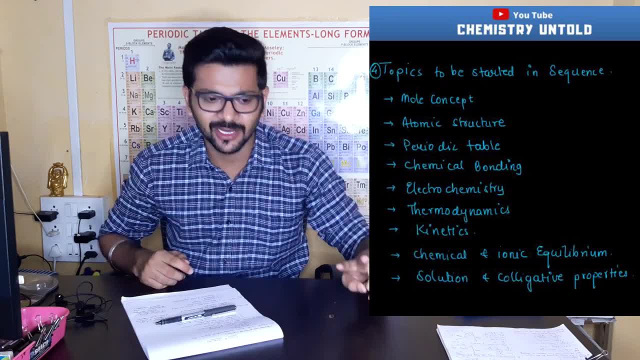 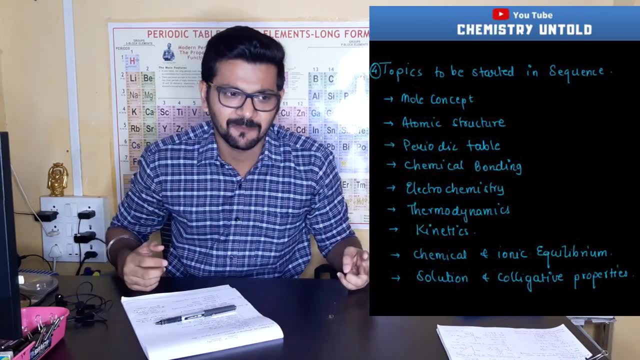 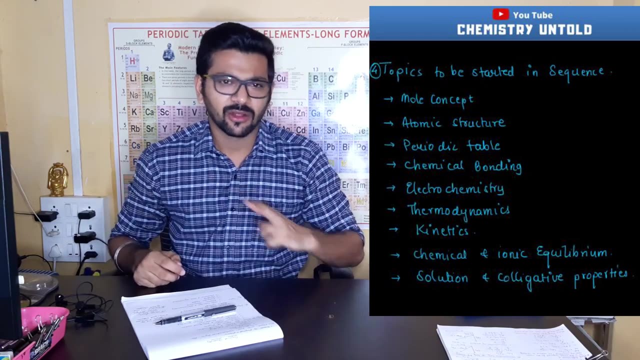 chemistry because mole concept in stoichiometry will involve a population. the numericals of mole concept and stoichiometry are quite tough. many times i see students from even master's level finding it difficult to solve stoichiometry and mole concept numericals or mcqs. start investing your time in atomic structure. i had all the formulas related. 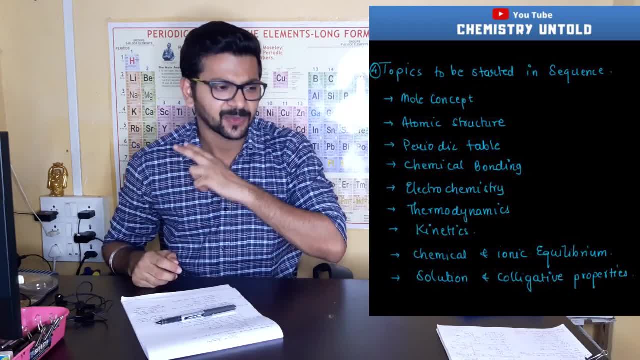 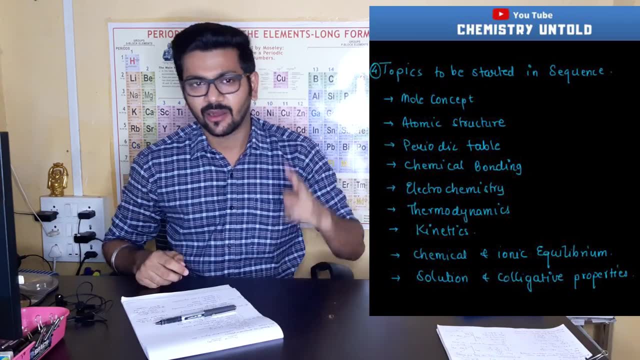 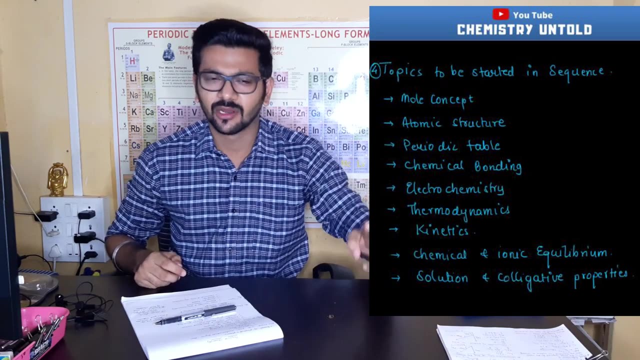 to boho's model, hydrogen spectrum, energy, radius, the theories, the electromagnetic radiation, the plank theory- and then getting into quantum chemistry, why there was a need for a quantum chemistry. now, understanding quantum chemistry will require a lot of physics. it will require a lot of information or knowledge about stationary wave, wave motion, circular motion and a standing. 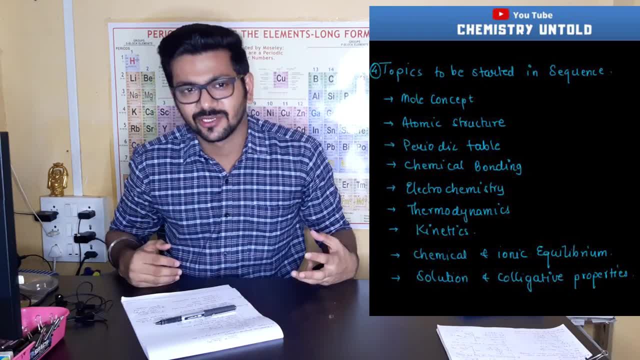 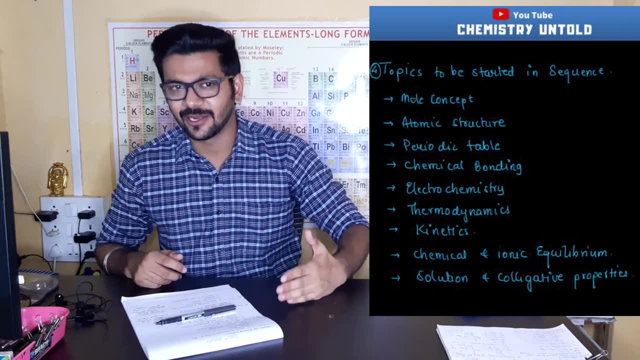 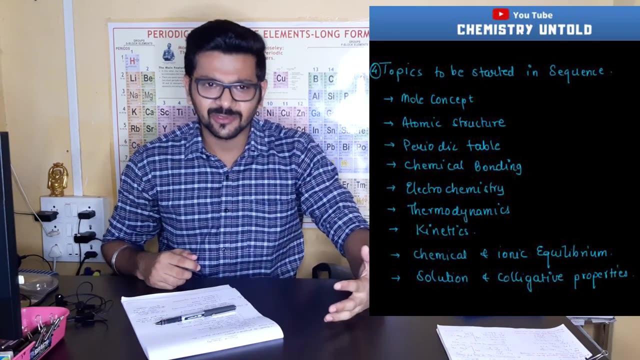 wave or you can say electromagnetic radiation. so start with atomic structure, then go with periodic table. once your periodic table is done, go with chemical bonding, because periodic table and chemical bonding are interrelated. hybridization, the geometry, vsepr theory, bonding, non-bonding orbitals, then molecular orbital theory, the shapes of molecular orbitals, and all those things once. 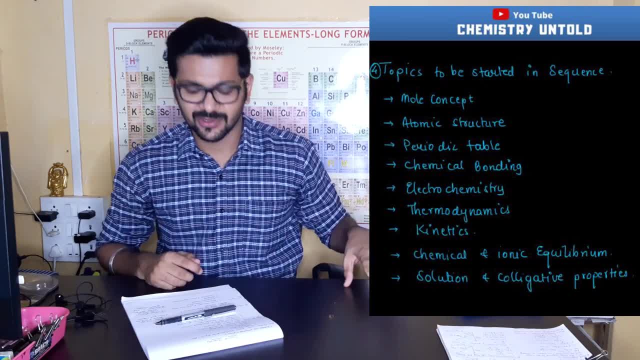 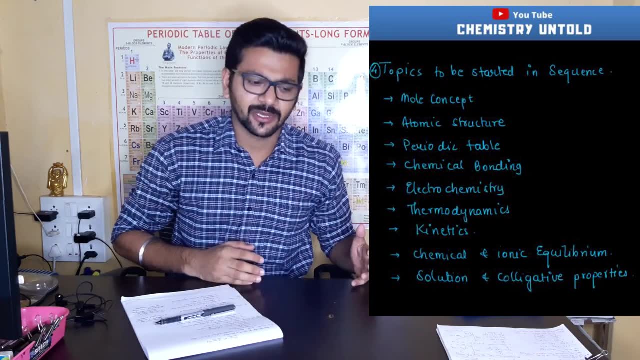 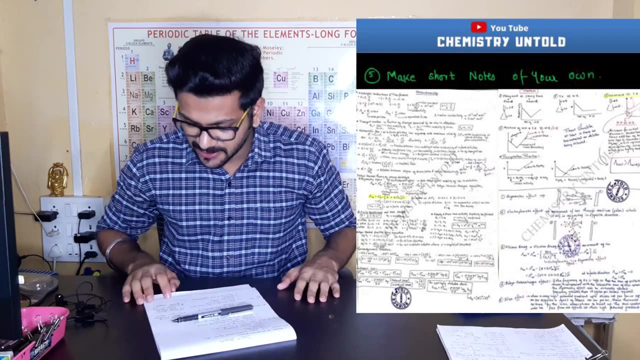 that part is completed, you are done with the initial part of physical chemistry. now you can start with chemical and ionic equilibrium, or any other topic, let's say chemical kinetics, electrochemistry, thermodynamics, because these three topics are going to play the most important, the crucial role in this training physical chemistry. so the fifth mantra that i can give you is: make. 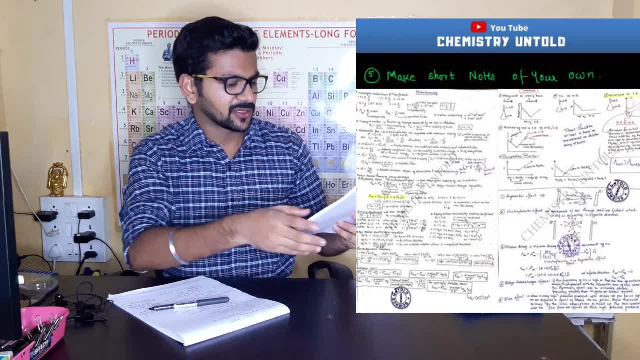 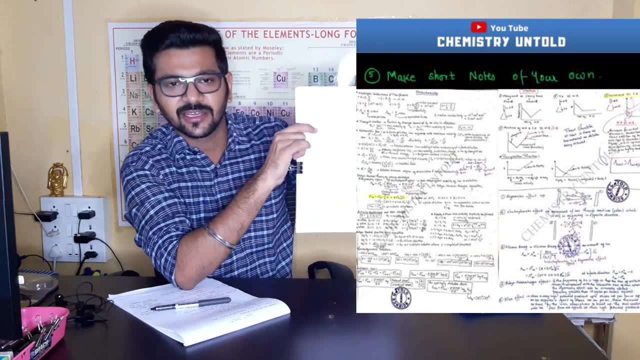 short notes. start making notes. as you can see over here, i have got this, i've got this. notes over here. you know this one paper and in this entire one paper i have written everything regarding zero order reaction that's from kinetics. so just a single sheet of paper and everything about chemical. 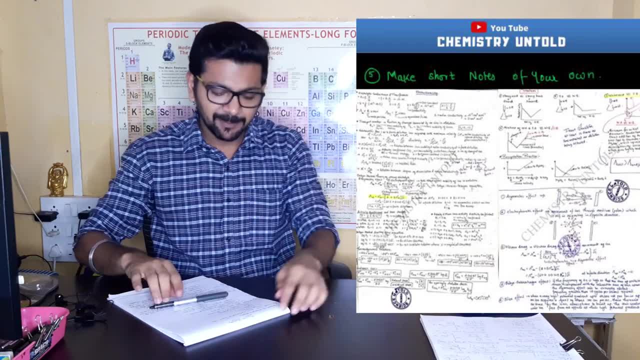 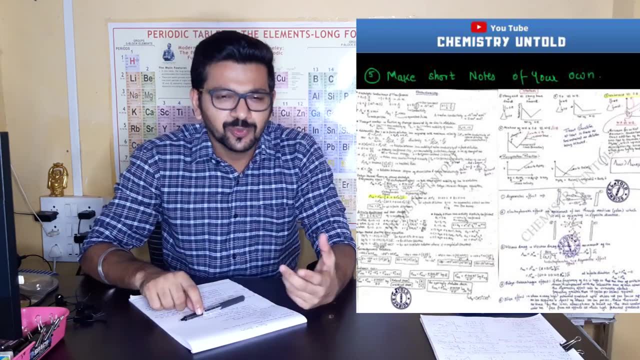 order. kinetics is done over here, but in your case what you can do is take a paper, write down all those important formulas, all those important unit conversions. you know, many times i've seen people asking me: so you provide us the notes. you know me, providing you notes will not serve the purpose. do.